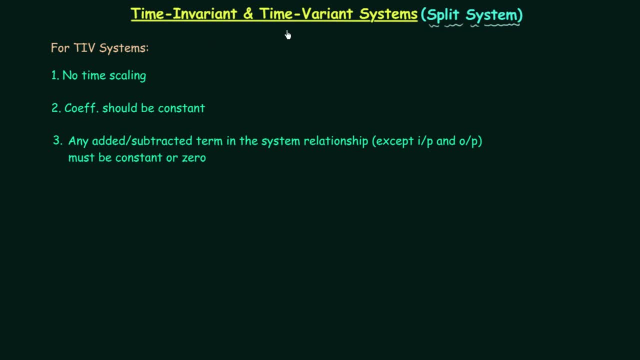 systems. we will find out if they are time invariant or time variant. So let's start with the first problem in this lecture, and the first problem is actually the fourteenth problem. till now we have completed 1 to 13th problem in the last two lectures and in this. 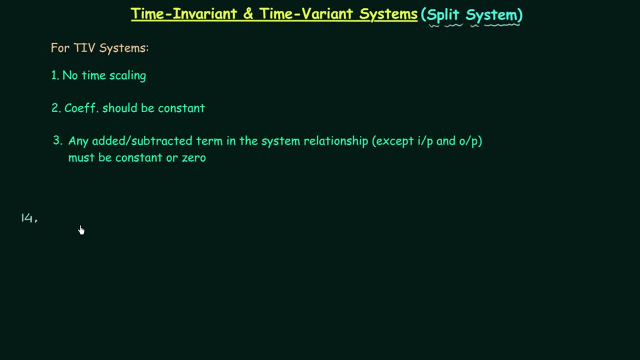 lecture we will discuss fourteenth and fifteenth problem, and the two problems are based on split systems. So let's see what is the relationship between input and output. Output yt is equal to xt minus 1 when time t is less than zero or negative, and it is. 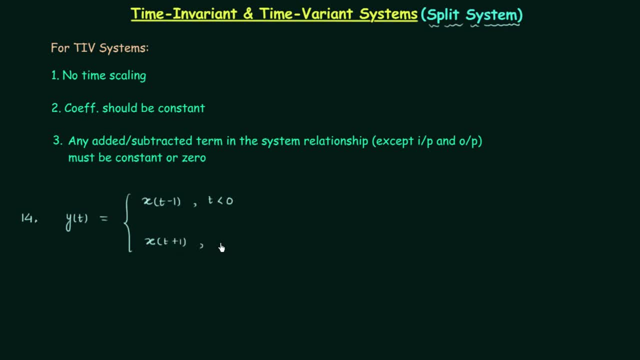 equal to xt plus 1 when time t is greater than or equal to zero. So when time t is zero or it is positive, yt is equal to xt plus 1, and when t is negative, yt is equal to xt minus 1.. So you can see, there is condition on time, there is condition on time and whenever there 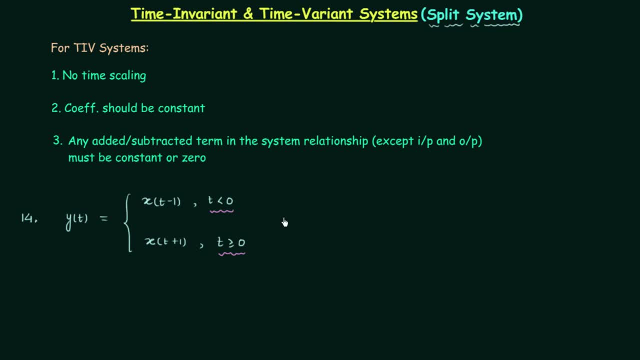 is condition on time. the system is known as split system. So this particular relationship is the relationship of split system and we are interested in finding out if this split system is time invariant or time variant. And for this, again, we will check the following conditions. 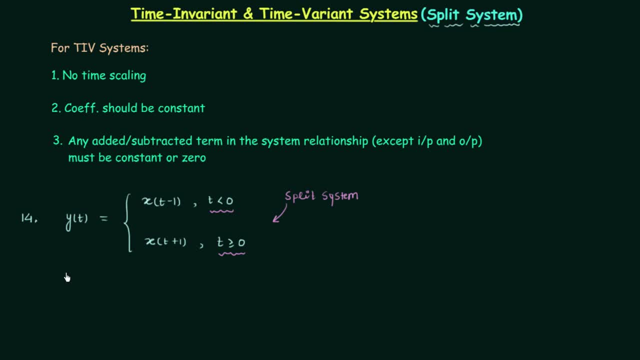 Let's see if the three conditions are true or not. We will start with the first condition. In the first condition we try to find out if there is any timescaling on the input side and also on the output side. On output side we only have t here, so there is no timescaling. 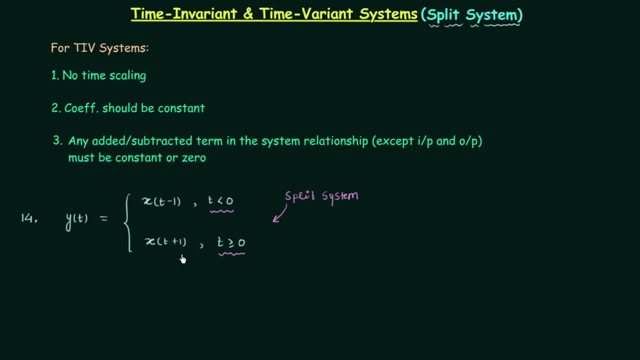 and on the input side you can see we have t minus 1 and t plus 1.. There is time shifting, no times scaling. So condition number 1 is true for this system relationship. Now we will check for condition number two. the coefficients should be constant. there are two coefficients. 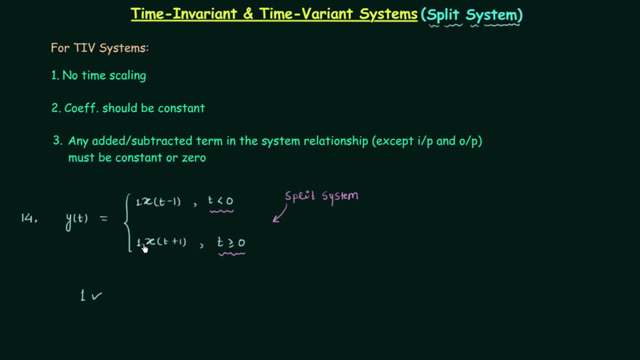 one here and one here. so the coefficients are constant. they are not function of time. so condition number two is also satisfied. now we will move to condition number three. any added or subtracted term in the system relationship, except input and output, must be constant or zero. here there is no added or subtracted terms. therefore condition number 3 is also satisfied. 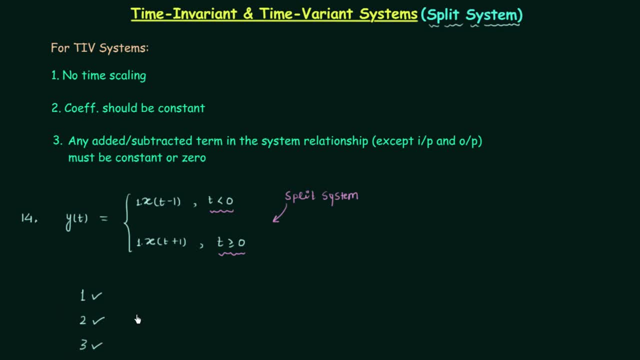 and as all the three conditions are satisfied, the system is time invariant system. you will say the system is time invariant system, but this answer is incorrect. the system is not time invariant, but it is time variant. and i will explain why. it is time variant by writing down time invariant by typing time Souстрons. 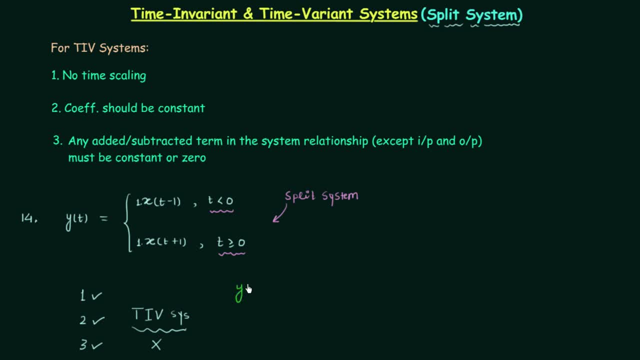 this system relationship. in some other form, yt is equal to at. x, t minus 1 plus bt, x, t plus 1, and here at and bt are defined like this: at is equal to 1 when t is less than 0, and it is equal to 0 when t is greater than or equal to 0. bt, on the other hand, is equal to 0 when t is less than. 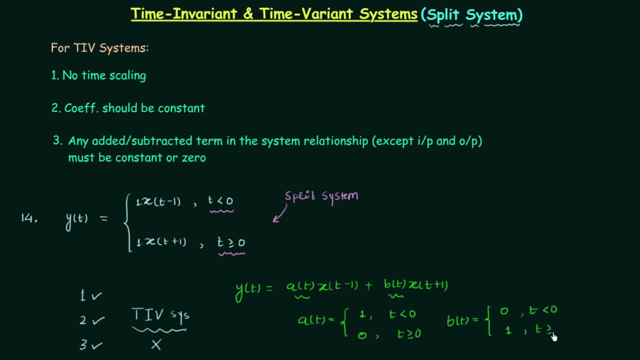 0 and it is equal to 1 when t is greater than or equal to 0. and if you try to compare the two system relationships, you will find they are same. in this case, when t is less than 0, yt is equal to x, t minus 1. and in this relationship, when t is less than 0, 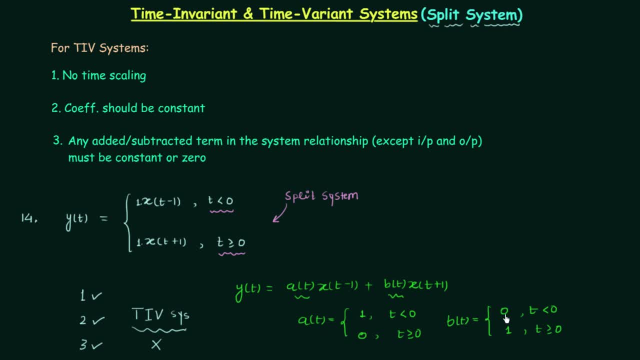 when t is less than 0, at is 1, but bt is 0, so this part will become 0 and we only have yt equal to x, t minus 1, as at is 1 and bt is 0. and when t is greater than or equal to 0, here yt is equal to. 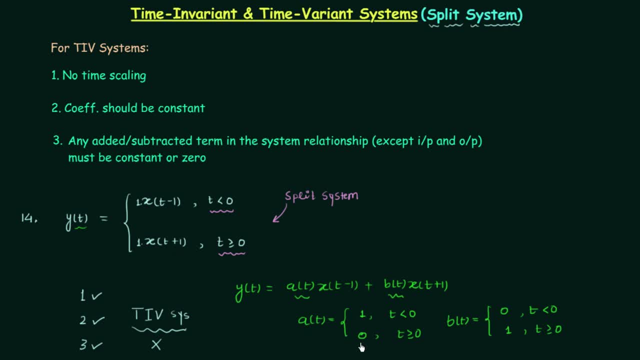 x, t plus 1. in this case, at will be 0, bt will be 1, at will be 0, bt will be 1, so yt will be x, t plus 1, so the two relationships are same and instead of writing it like this, we can write it like this, and you can clearly see we have two coefficients. 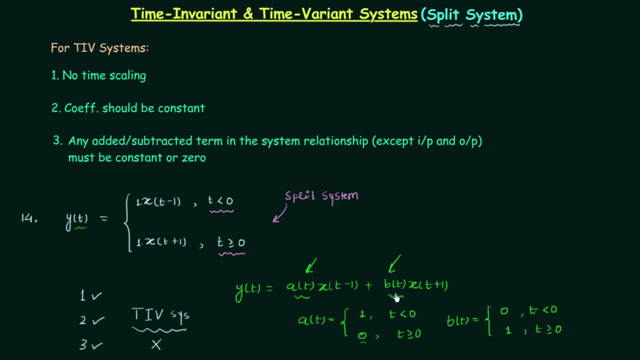 at and bt. they are the two coefficients and according to condition number two the coefficients should be constant. but here at is not a constant coefficient and also bt is not a constant coefficient. they are time dependent. they depend on time. you can see the definitions. they depend on time. so we can say that condition number two is violated.